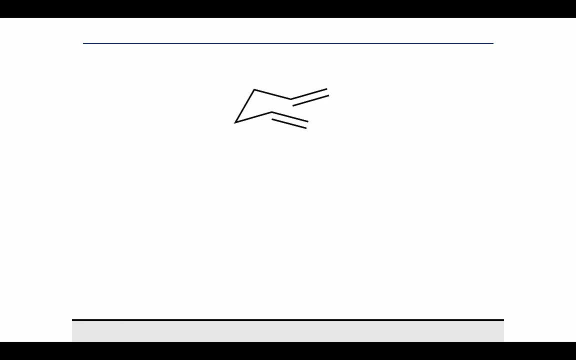 Thank you for joining us on Synthesis Workshop. In today's installment of our Advanced Organic Chemistry course, we're joined by Riya Halder. Riya earned her bachelor's with honors in chemistry at Hindu College University of Delhi. She subsequently completed her master's. 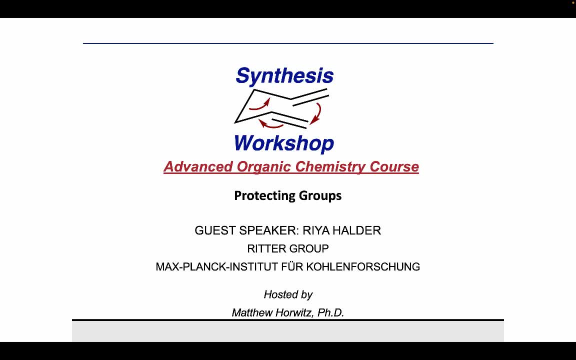 at the Indian Institute of Technology, Delhi, where she worked under the supervision of Dr Nidhi Jain. Currently, she's pursuing her PhD at the Max Planck Institute in the group of Professor Tobias Ritter. Today, Riya will give us a lecture on protecting groups. 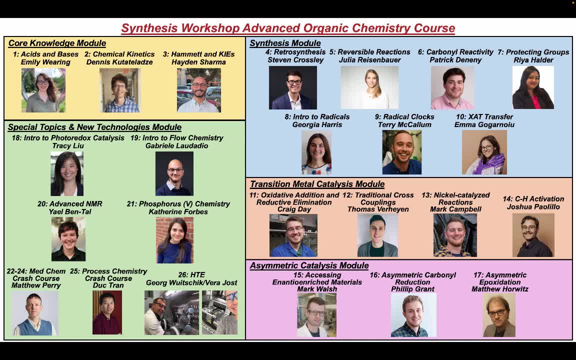 which we'll see have been a cornerstone in allowing chemoselective operations to be carried out in organic synthesis. And from there I'll let you get started, Riya. Thank you very much for joining us as a guest speaker today. Thank you, Matt, for the kind introduction and for inviting me to this platform. The 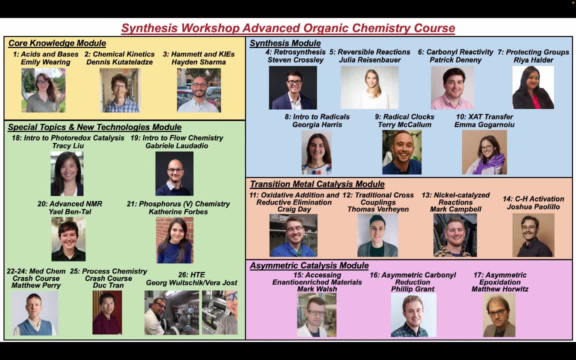 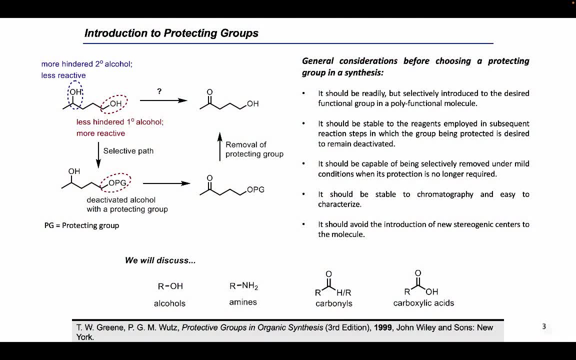 topic that I'll be talking about in today's Advanced Organic Chemistry course is the multi-step organic synthesis. In the planning and execution of such multi-step synthesis, an important consideration is the compatibility of the functional groups that are already present with the reaction conditions required for subsequent steps. It is frequently necessary. 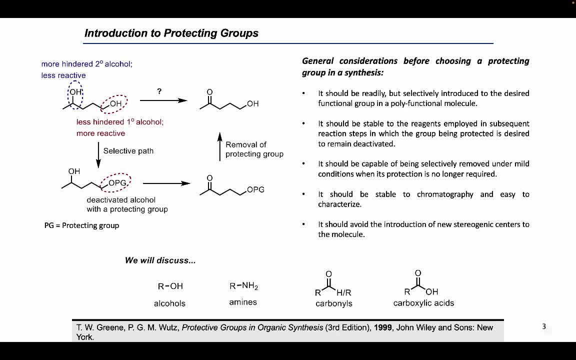 to modify a functional group in order to prevent interference with some reaction in the synthetic sequence. A protecting group is a molecular framework that is introduced onto a specific functional group in a polyfunctional molecule to block its reactivity under reaction conditions needed to make modifications elsewhere in the molecule. Three basic questions to 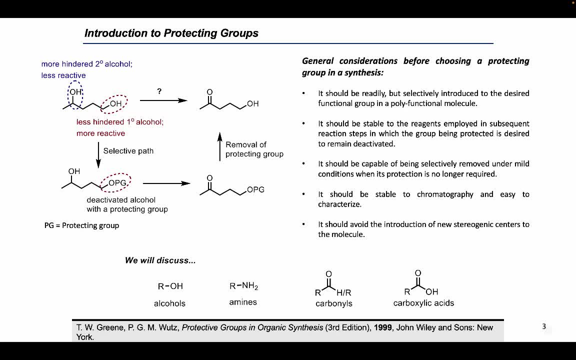 address when choosing a protective group are: Can I put it on where, and only where, I want? Will it survive all future reaction conditions and will it affect the reactivity of the substrate? And can I take it off, and only it off when needed? It is also a fact that each protecting group incorporated in a multi-step synthesis increases. 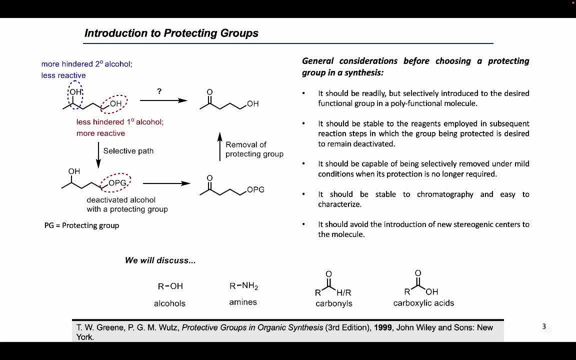 the number of steps to the synthesis and reduces the overall yield and efficiency. Fortunately, the methods of protective group installation and removal have been highly developed and the yields are usually excellent. This episode presents information on the synthetically useful protective groups for four major functional. 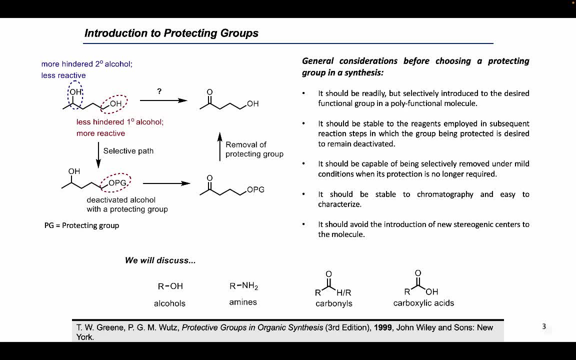 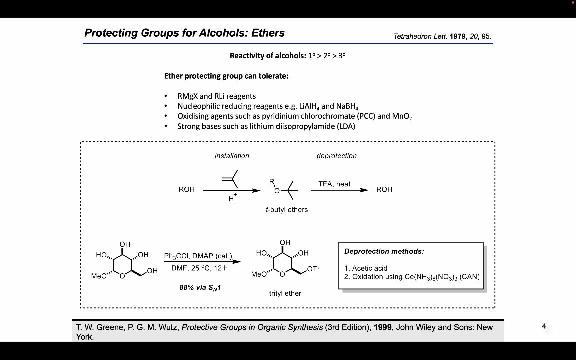 groups- ie the hydroxy group, the amine group carbonyl group- ie aldehydes and ketones, and the carboxylic acid groups. Ethers are one of the most important protecting groups for alcohols. All ethers are stable to basic reaction conditions and can tolerate. 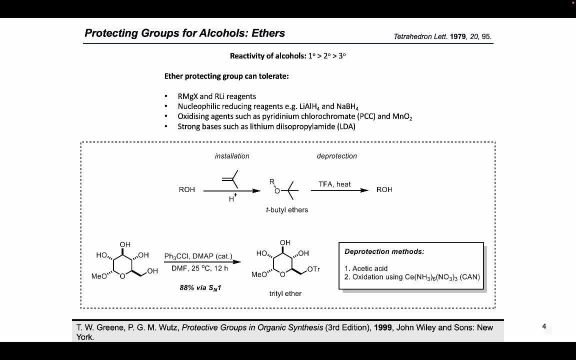 organometallics like lithium-aluminium hydride and sodium borohydride, and even oxidizing agents such as pyridinium chlorochromate and manganese dioxide. Also, they are stable to very strong bases such as LDA, The simple alkyl groups like methyl ethers, which are readily 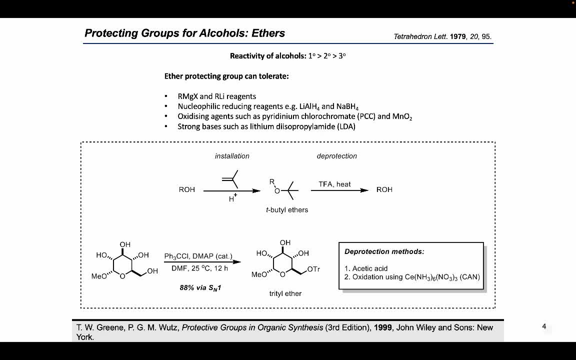 accessible via the Williamson ether synthesis are generally not very useful for protection of alcohols because they require very harsh electrophilic conditions for deprotection. The third butyl group is an exception and has found some use as a hydroxy-protecting. 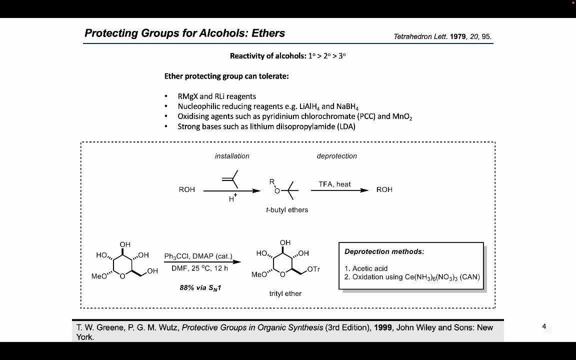 group Owing to its stability of the third butyl cation. third butyl ethers can be cleaved under moderately acidic conditions. The third butyl group is normally introduced by reaction of the alcohol with isobutylene in the presence of an acid catalyst, The third butyl group is removed under even milder conditions. 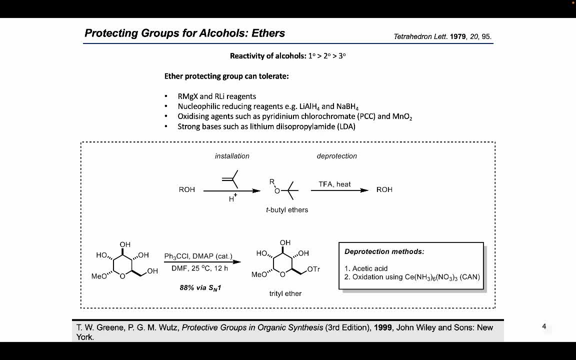 and is an important hydroxy-protecting group, especially in carbohydrate chemistry. This group is introduced by reaction of the alcohol with triphenylmethyl chloride via an SN1 cell. Hot aqueous acetic acid suffices to remove the third butyl group. The ease of removal 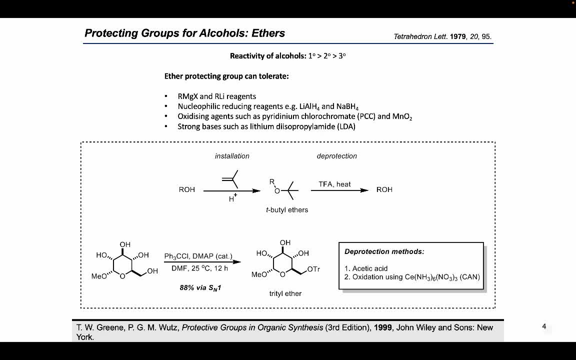 can be increased by addition of electron-donating substituents. Third butyl groups can also be removed oxidatively using ceric ammonium nitrate In case a molecule cannot tolerate the acidic conditions required for cleavage of an ether-protecting. 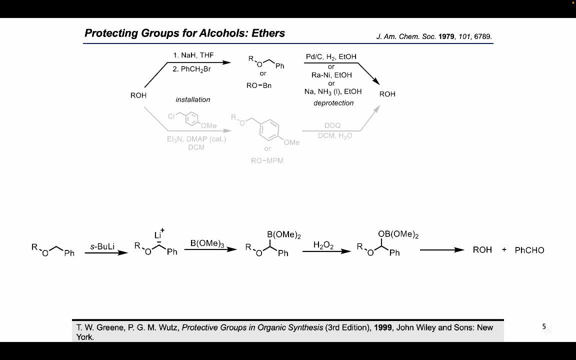 group, the benzyl group, can serve as a hydroxy-protecting group as they are quite stable to the point where they can be removed. The third butyl group can be removed by addition of an electron-donating substituent, The benzyl. 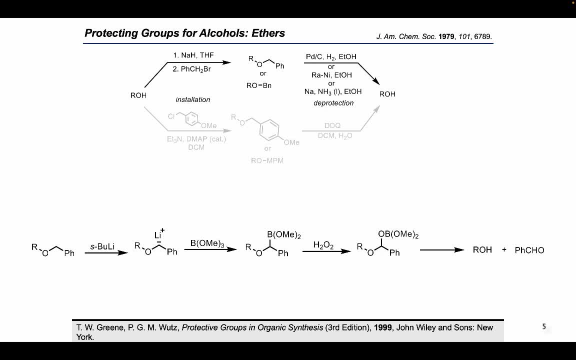 group can serve as a hydroxy-protecting group as they are quite stable to the point where they can be removed In case a molecule cannot tolerate the acidic conditions required for cleavage of an ether-protecting group. the benzyl group can serve as a hydroxy-protecting group as they are quite stable under both. 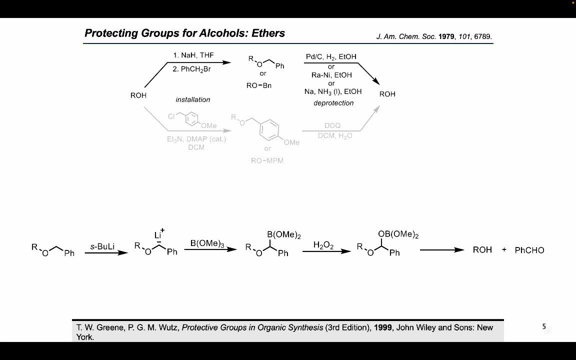 acidic and basic conditions, and also toward a wide variety of oxidizing and reducing reagents. Benzyl groups are usually introduced by the Williamson reaction. Catalytic hydrogenolysis offers the mildest method for deprotecting benzyl ethers. Butyllithium. 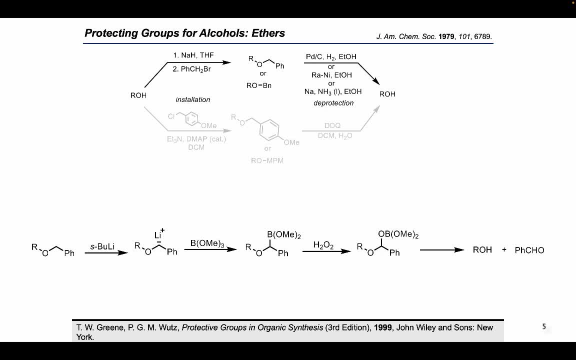 can be used to deprotonate a benzylic hydrogen. Therefore, the lithiated ether obtained by the treatment with SN1 and SN2 can be used to deprotonate a benzylic hydrogen. Therefore, the lithiated ether obtained with S-butyllithium forms alkyl boronate by reaction with trimethyl. 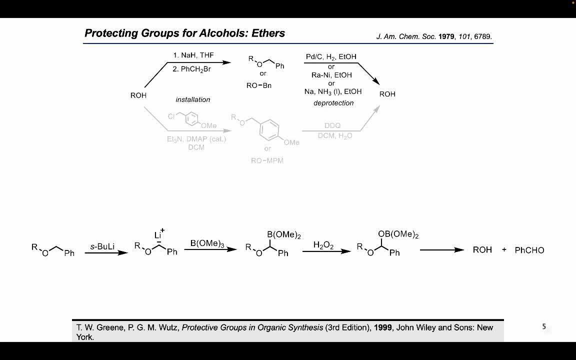 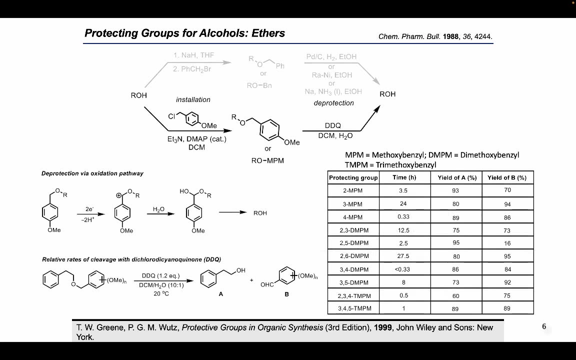 borate. And then finally, oxidation with hydrogen peroxide liberates the unmasked alcohol. Hydrogenolysis of secondary and tertiary benzyl ethers can be sluggish. Protection of alcohols using benzyloxy-methyl chloride produces corresponding methoxybenzyl ethers, which are cleaved more. 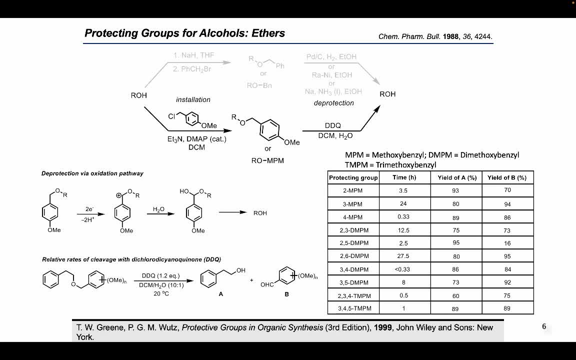 readily than the corresponding methoxybenzyl ethers. These groups can be removed oxidatively by using DDQ. The reaction proceeds through a benzylic cation and the methoxy substituent is necessary to facilitate the oxidation. The ease of removal can be increased by further addition of methoxy group, as is summarized. 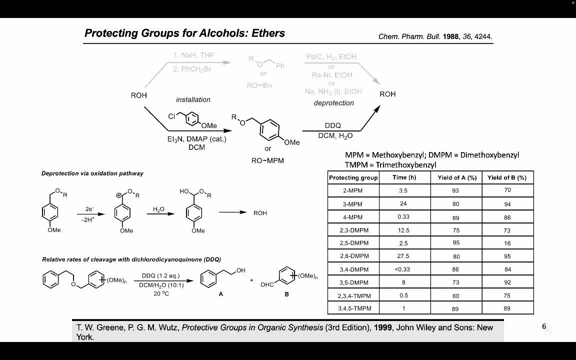 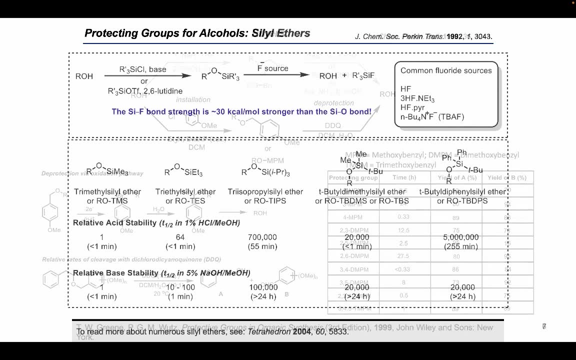 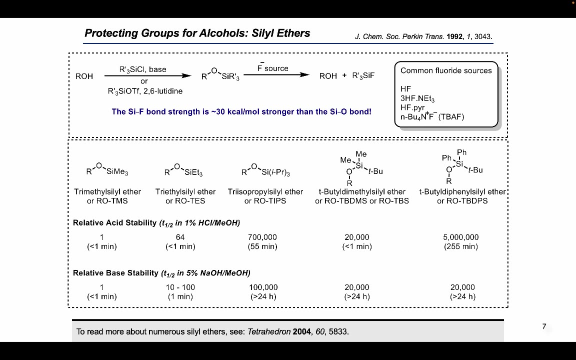 in the rate of cleavage table. These reaction conditions do not affect most of the other common hydroxyprotectants. Silyl ethers are among the most frequently used protective groups for the alcohols. This is because their reactivity, that is, both formation and cleavage, can be modulated by. 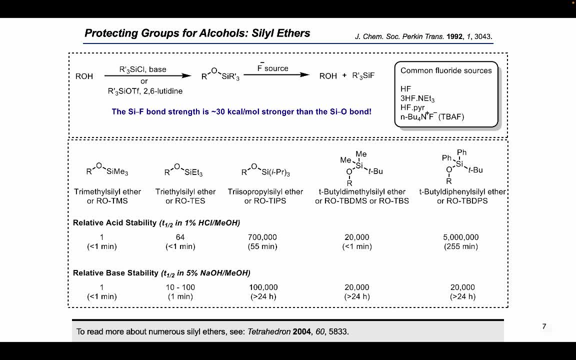 a suitable choice of substituents on the silicon atom. Both steric and electronic effects regulate the ease of cleavage in multiply functionalized substrates and hence should be considered in planning the selective T protection. Alcohols can easily be converted to silyl ethers by reaction with trialkyl silyl chlorides. 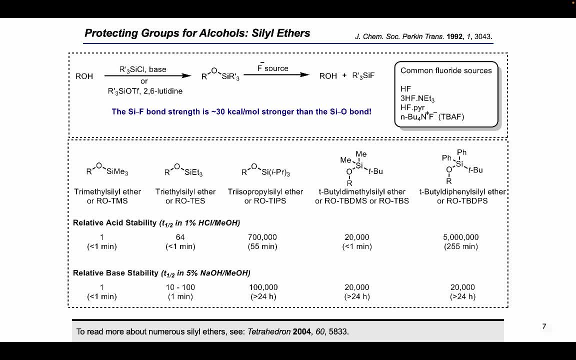 in presence of an amine base. Also, they are easily cleaved by exposure to fluoride ion, which is attributed to the high affinity that fluoride ion has for silicon. The reported half-lives vary as a function of environment and acid or base concentration, but they serve. 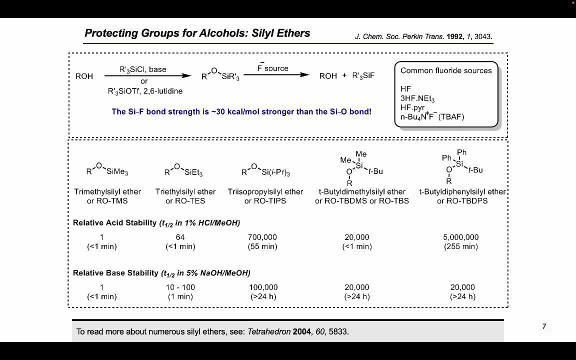 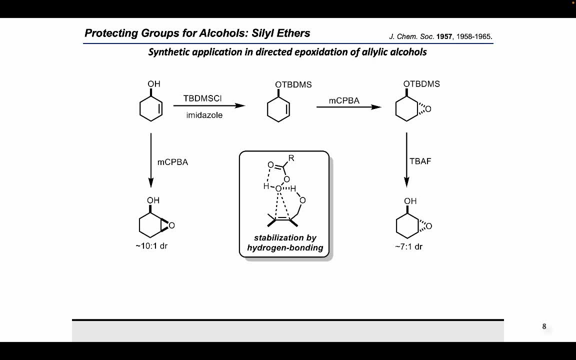 to help define the relative stability of these silyl groups. One of the applications of silyl ethers is in the epoxidation of allylic alcohols that showed facial selectivity when using MCPBA oxidant, in which hydrogen bonding played a. 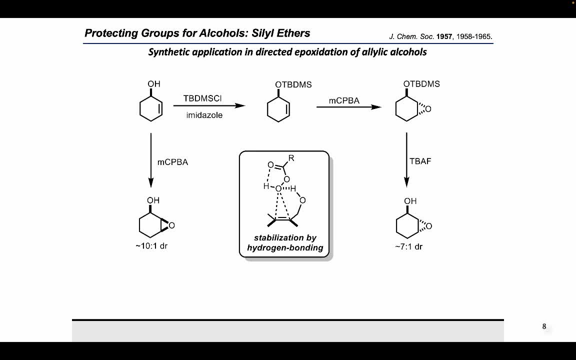 key role. The hydroxy group can form hydrogen bond with the oxygen in the epoxide, stabilizing it, and hence prefers to add the epoxide to the same phase as the hydroxy group. However, when the hydroxy group is masked using bulky TBS group steric effects, direct peroxide, addition to the opposite phase of the hydroxy. 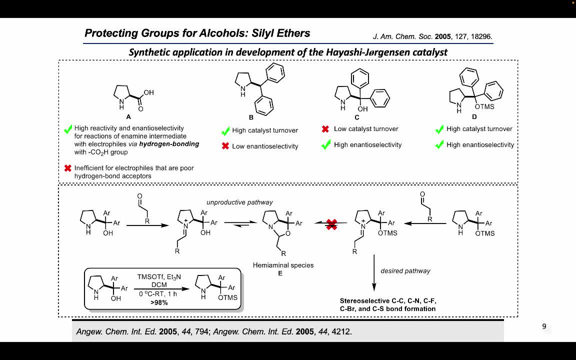 group. Another novel application of silyl ethers is found in the development of the Hayashi-Jogerson catalyst. Proline, often referred as a universal catalyst, is certainly a part of this noble club because of its high utility in the enantio-selective transformations of aldehydes. However good 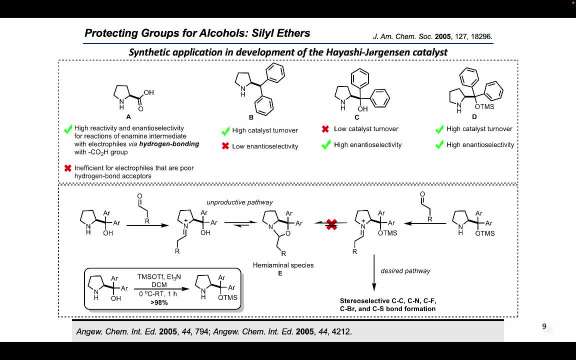 hydrogen bonding properties of the electrophiles is required to achieve high asymmetric induction. In 2005,, after carrying out a careful survey, Hyaluronic Acid was found to be the most effective solution for the hydroxy group. In 2005,, after carrying out a careful survey, Hyaluronic Acid was found to be the most effective. 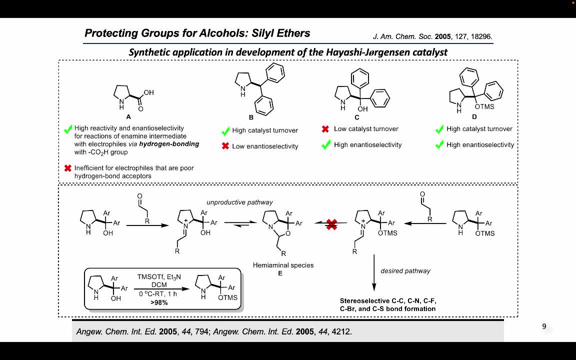 solution for the hydroxy group. In 2005,, after carrying out a careful survey, Hyaluronic Acid was found to be the most effective solution for the hydroxy group. The coses of hydroxy group independently became a input of pyrolidine derivatives that could potentially 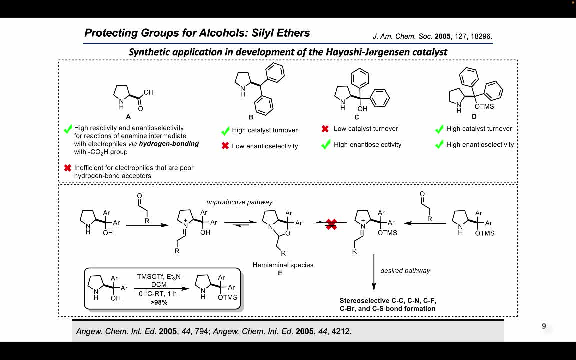 of hydroxy group independently came up with a set of pyrolidine derivatives that could overcome the previous limitations. Structure B in the present slide was found to be a highly active catalyst for a variety of transformations, but very low enantio-selectivity obtained. 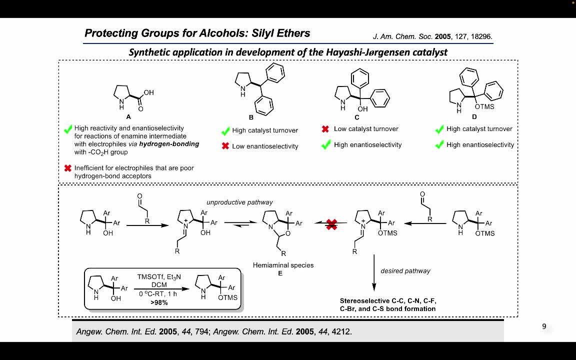 On the other hand, structure C provided reactions with a very good level of stereocontrol but a low catalyst turnover, which was attributed to the formation of a relatively stable and unreactive hemi-aminal species E. To prevent this, the hydroxyl group was protected with 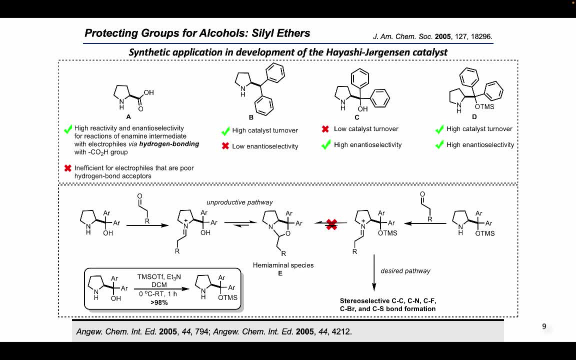 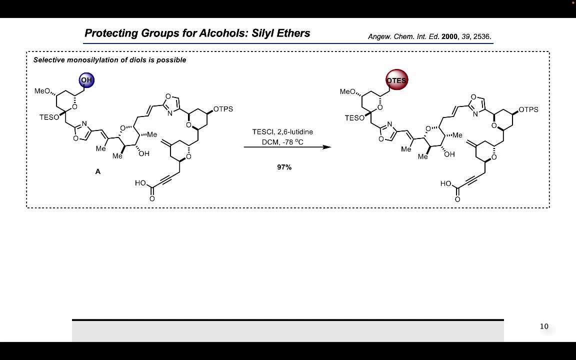 a TMS group which could be repaired in a single step with a very high yield. This simple modification substantially increased the catalytic turnover in the alpha functionalization of aldehydes. We have seen that one of the requirements of good protecting group is that it should be readily 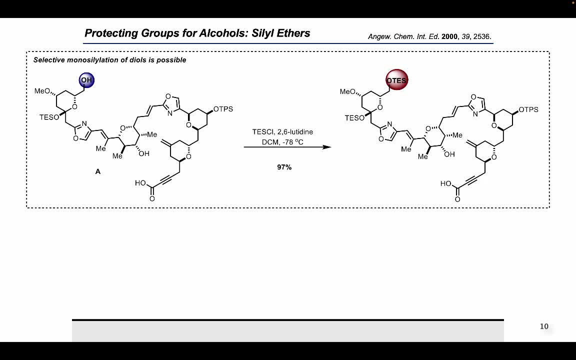 and selectively introduced to the desired functional group in a polyfunctional molecule, and also should be capable of being selectively removed under mild conditions when its protection is no longer required. Attempts were made to selectively cellulate the primary hydroxyl group of the molecule A, A combination of TESC. 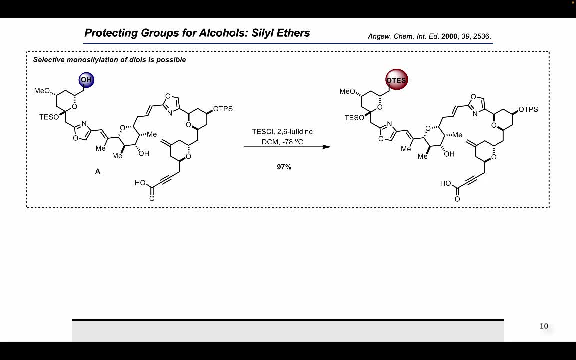 L and imidazole resulted in a mixture of base cellulation of both the carboxyl and secondary hydroxy groups. Ultimately, a change in the base from imidazole to 2,6-lutidine led to an exclusive cellulation of the desired primary hydroxyl group. The difference in the selectivity 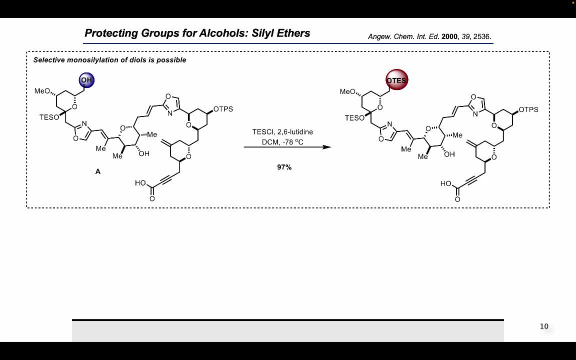 between the two bases is presumed to be a result of the formation of a more active cellulating agent. aside from the reaction of imidazole with the silyl chloride, Apparently there is no reaction between the silyl chloride and 2,6-lutidine, which simply acts as a base. 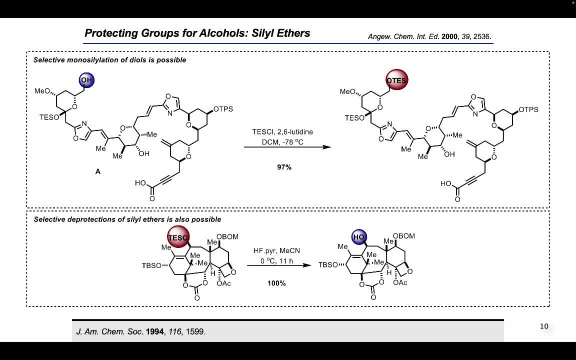 Also, we have learned that the steric factors play an important role in determining selectivity of deprotection of silyl ethers. As a result, the TES ether can be cleaved in the presence of a bulkier TBS ether using HF-inertia. 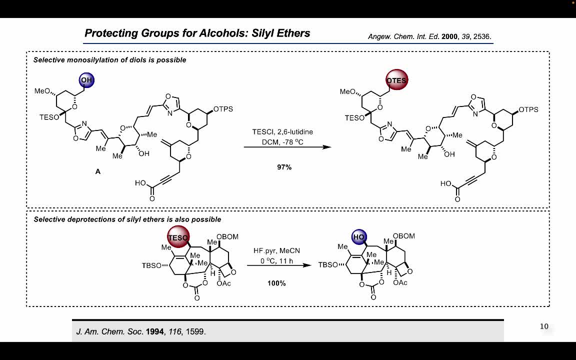 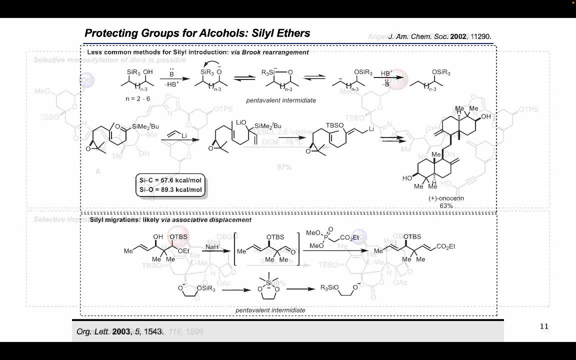 In general, methods used to cleave the TBS ether are effective for cleavage of the TES ether. A less common method to prepare silyl ethers is via Bruch rearrangement, which involves an intramolecular migration of a silyl group from carbon to oxygen in. 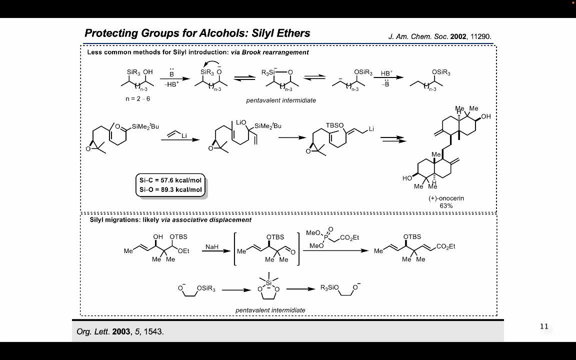 presence of a catalytic amount of a base, A cyclic pentavalent silicon species is formed after deprotection of silyl ethers. in the presence of a catalytic amount of a base, A cyclic pentavalent silicon species is formed after deprotection of a base. A cyclic pentavalent silicon species is formed after deprotection of a base. 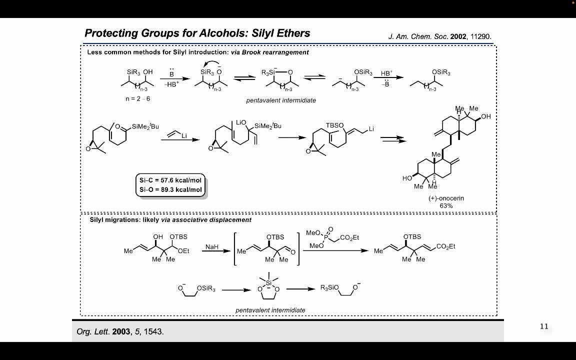 Subsequent ring opening and fast and irreversible protonation of the carbon ion leads to the corresponding silyl ether. The greater strength of a silicon-oxygen bond as compared to the silicon-carbon bond provides the driving force for the conversion, The ability to migrate. 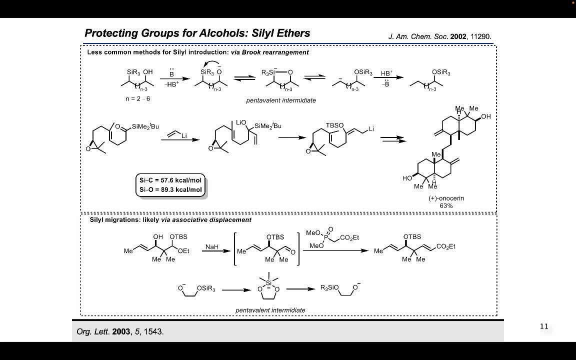 from one hydroxyl to another is another property of silyl ethers that can be used to advantage, under basic conditions, in protic solvents and proceed intramolecularly through a penta-coordinated silicon. The concept was used advantageously in Overman's synthesis of L-cyanine, in which 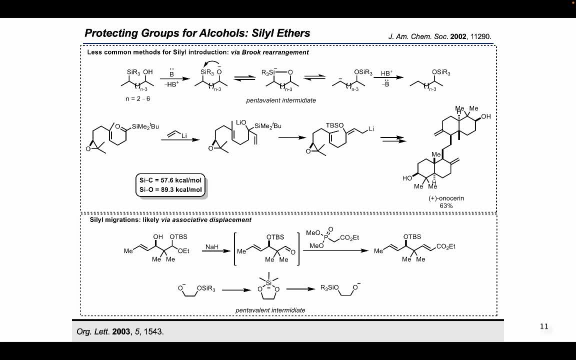 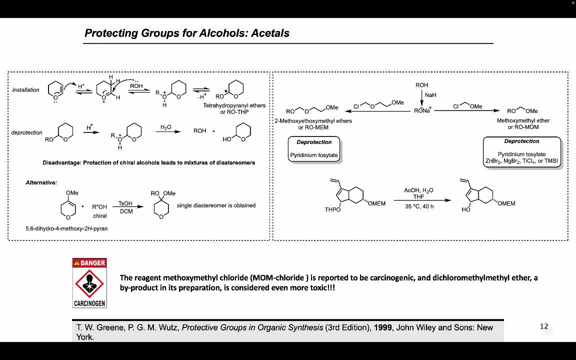 silyl migration facilitated the deprotection of a hindered TBS ether. Another class of protecting groups used for alcohols is acetyls and ketols. These are also inert to basic and nucleophilic reagents and remains unchanged under hydride reduction and organometallic reactions. It also 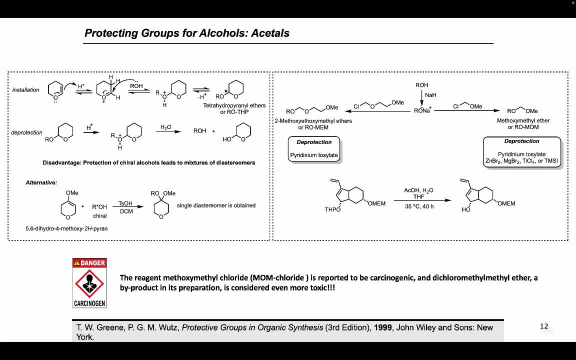 protects the hydroxy group against oxidation. The tetrahydropyroneal ether, or the THP group, is applicable. when mildly acidic hydrolysis is appropriate for deprotection, It is introduced by an acetate. One way of avoiding this problem is to use 5,6-dihydroformethoxypyrene where no new 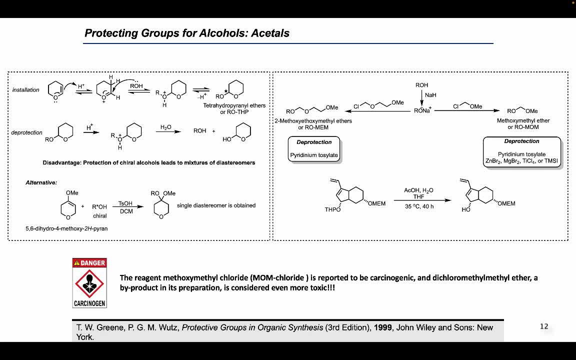 catalysts are used. Alpha-haloethers are also often used for the protection of alcohols. Their high reactivity in nucleophilic displacement reactions by alkoxides permits protection of alcohols under mild conditions. The MOM and mem groups are normally introduced by reaction of an. 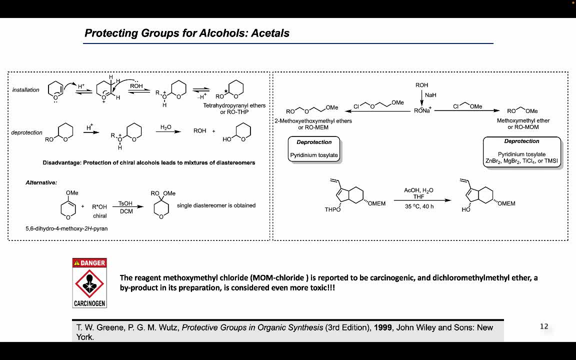 alkali metal salt of the alcohol with methoxy methyl chloride or methoxy ethoxy methyl chloride. The MOM and MEM groups are also used for the protection of alcohols. under mild conditions, and MEM groups can be cleaved by pyridinium tosylate. 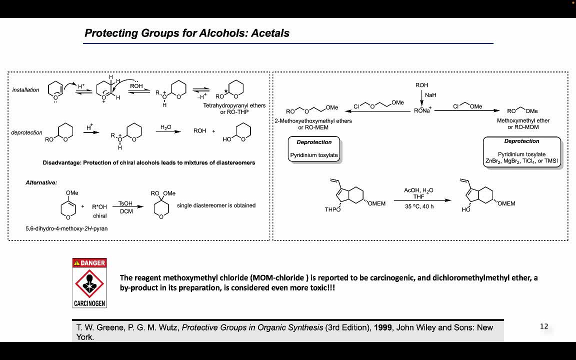 The MEM group can easily be removed under non aqueous conditions, and reagents such as zinc bromide, magnesium bromide, titanium tetrachloride or trimethyl silyl iodide permits its removal. The MEM group is more stable to acidic aqueous hydrolysis than the THP or the MOM group. 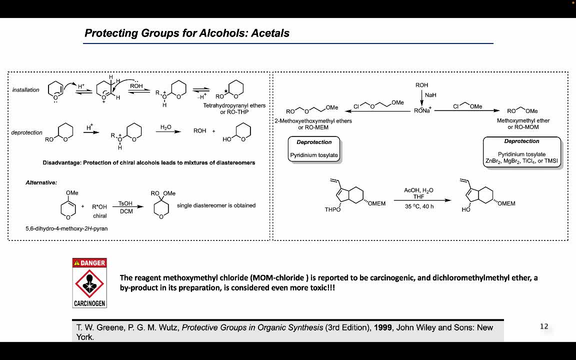 This relative reactivity relationships allow the THP and MEM groups to be used in a complementary fashion when two hydroxy groups must be deprotected at different points in a synthetic sequence. Please note that the use of MOM chloride to protect alcohols is associated with a big 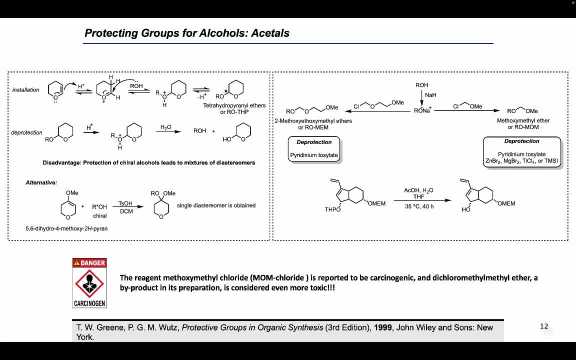 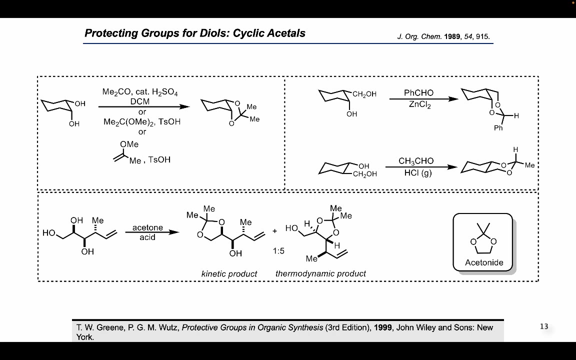 safety concern, as the reagent is highly carcinogenic to humans and the by-product formed during its preparation is even more toxic. Special precautions must be taken when using such chemistry, especially during a large-scale synthesis. Acetylization of 1,2 and 1,3-diols plays an important role in manipulating the reactivity. 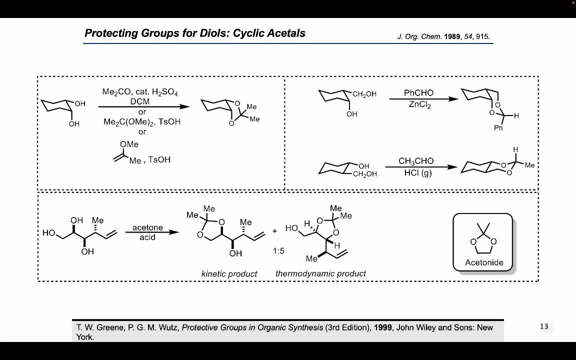 of cyclic and acyclic polyhydroxy compounds. Acetyls of 1,2 and 1,3-diols are readily accessible from their reactions with aldehydes in presence of an acid catalyst. Once formed, they are easily removed from the body. 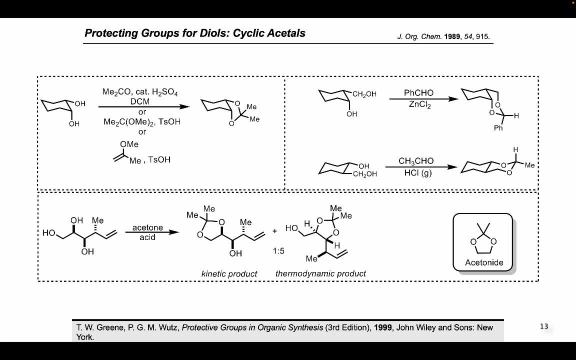 Once formed, these acetyls are very stable to basic conditions, but are labile towards acids. In preparing acetonides of triols, the 1,2-derivative is generally favoured over the 1,3-derivative, which in turn is favoured over the 1,4-derivative. 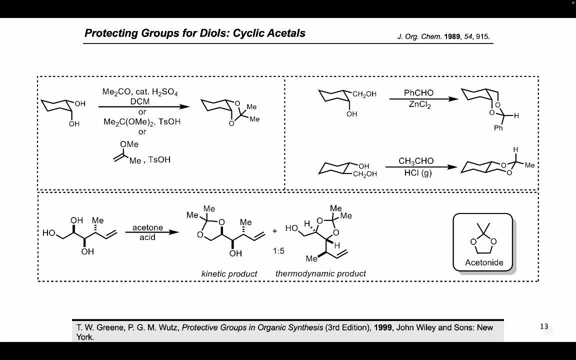 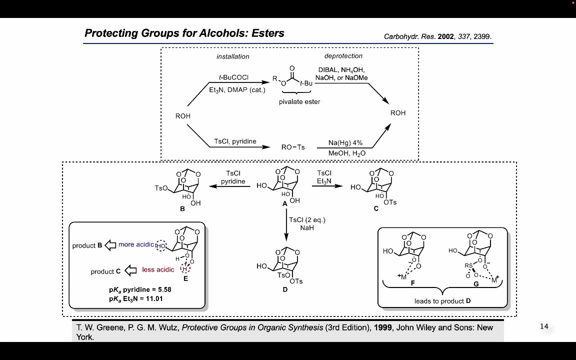 In cases where two 1,2-acetonides are possible, the thermodynamically more favoured one prevails and the secondary alcohols have a greater tendency to form cyclic acetyls. Protection of an alcohol functional group by esterification sometimes offers advantages. 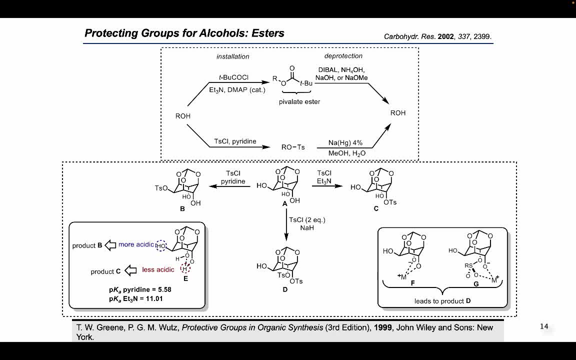 over use of acetyl or ether groups, because generally esters are stable under acidic conditions and are especially useful in protection during oxidations. Third, butanoyl esters, also known as the pylolid esters, can easily be prepared from alcohols. 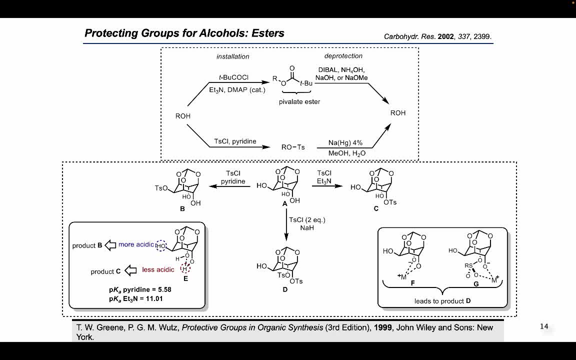 by reaction with pylol. The pylolid esters can be prepared by using pylol chloride in presence of a base and D-MAP as catalyst to increase the reaction rate. The steric bulk of the terbutyl group makes these esters resistant to nucleophilic attack. 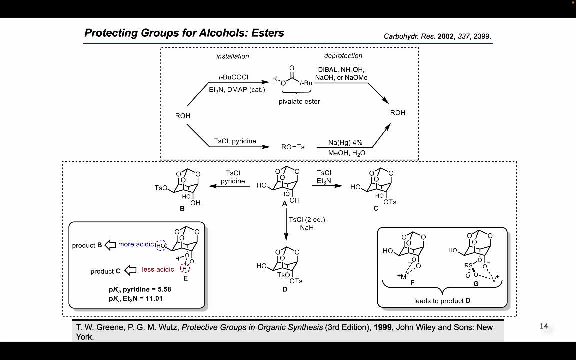 including hydrolysis, under mild basic conditions. Paraetolene sulfonate esters are often used for the regioselective protection of hydroxyl groups in carbohydrates and nucleic acids. Methods for the selective deprotection of hydroxyl groups. 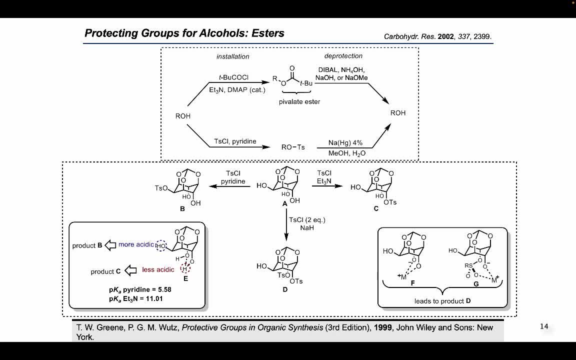 Methods for the selective deprotection of hydroxyl groups. The deprotection of hydroxyl groups include reductive cleavage with sodium, mercury amalgam and methanol solution. Also with the tosyl protecting group, some interesting selectivity has been obtained. 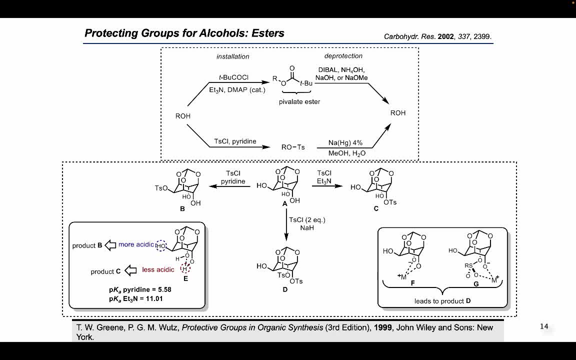 The different regioselectivity observed for the sulfonylation of triol-A in the presence of pyridine and triethylamine is due to the difference in their basicity. Triethylamine, being a stronger base, can deprotonate one of these esters. 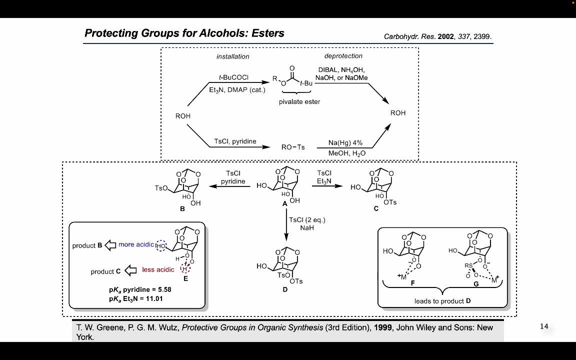 chez Mara Louboutin. direct flow of unethyl hydroxychloride in tosyl hydroxyl groups whose acidity is lower than that of the equatorial hydroxyl group due to a very strong intramolecular hydrogen bond. 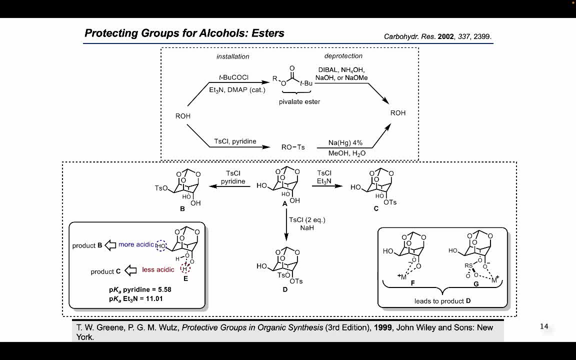 Since the equatorial hydroxy group is more acidic, sulfonylation takes place at this position in pyridine. Moreover, preferential titosylation of the axial hydroxyl group in presence of estudio du deμο from the facile chelate formation with the metal ion, as shown in the structure F and G. 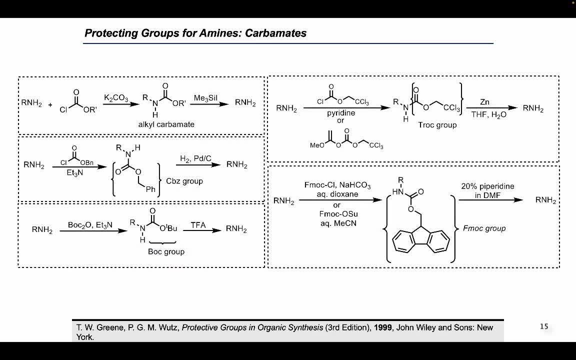 The second functional group that I am going to talk today is about amines, which are nucleophilic and easily oxidized. Primary and secondary amino groups are sufficiently acidic that they are deprotonated by many organometallic reagents, If these types of reactivity are. 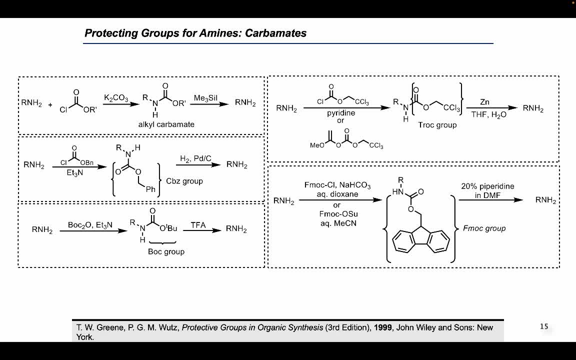 problematic. the amino group must be protected. The most general way of masking nucleophilicity is by acylations, and carbamates are particularly useful. Treatment of primary and secondary amines with alkyl chloroformate in presence of a base furnishes the corresponding alkyl carbamates. 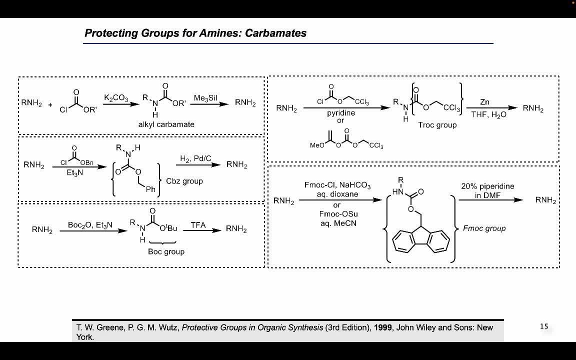 They are stable to oxidizing agents and aqueous bases and may be react with reducing agents. Iodotriene Trimethylsilane is often used for the removal of the protecting group. Another carbamate protecting group is the troch group that can be reductively cleaved by zinc. 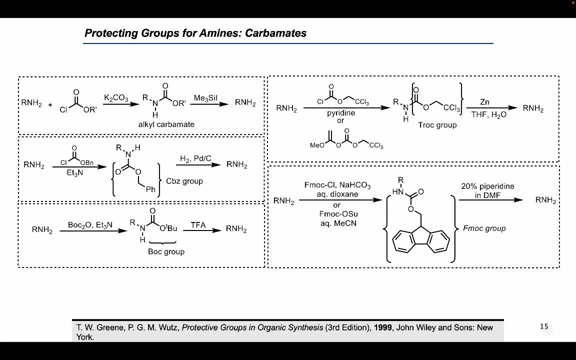 Under these conditions, the troch group can be cleaved in the presence of the BOK and the benzyl groups, about which I am going to talk soon. Next is the CBZ group, which is one of the most important nitrogen protecting groups in organic synthesis, especially in the peptide synthesis. 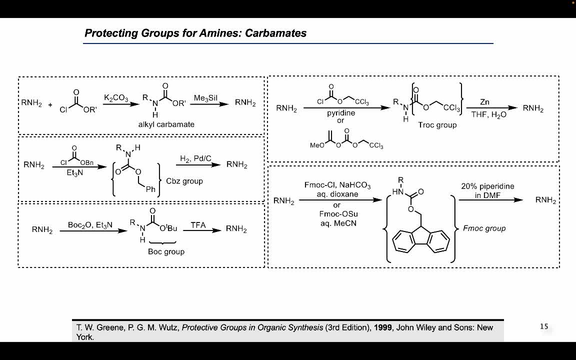 It is introduced by reacting the amine with benzyloxycarbonyl chloride in presence of a base. The protected amine is stable to both aqueous acid and bases and can be removed by hydrogenolysis. The BOK group is another widely used protecting group for primary and secondary amines. 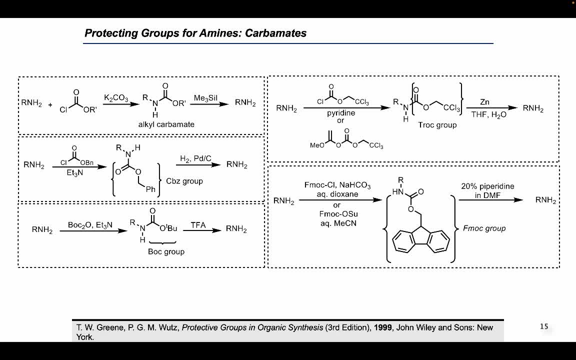 It is inert to hydrogenolysis and resistant to bases and nucleophilic reagents, but is more prone to benzyloxycarbonyl chloride. It is more prone to cleavage by acids than the CBZ group. Deprotection of the BOK group is conveniently carried out with TFA. 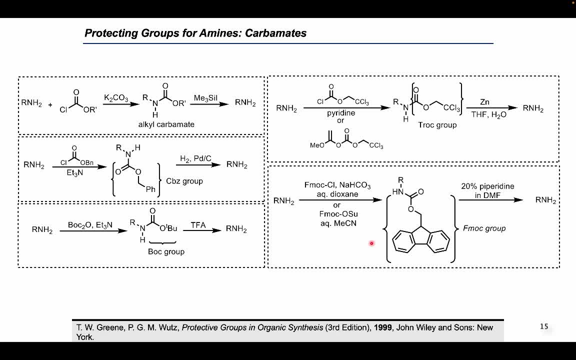 Another frequently used protecting group for amines is F-MOG carbamate, which can be introduced by reacting the amine with fluorenyl methyl oxy, carbonyl chloride. Piperidine is usually preferred for F-MOG group removal as it forms a stable adduct with the dibenzofluvene by-product. 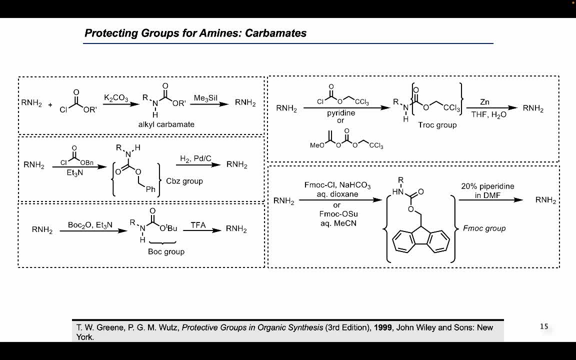 preventing the formation of a stable adduct with the dibenzofluvene by-product. preventing the formation of a stable adduct with the dibenzofluvene by-product. preventing the formation of a stable adduct with the dibenzofluvene by-product. preventing it from reacting with the substrate. 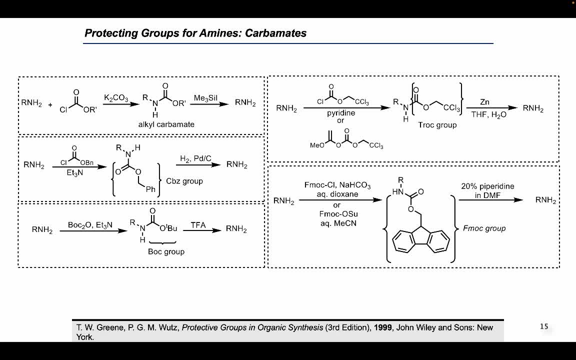 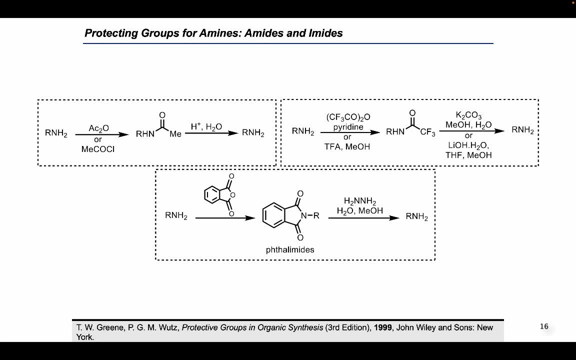 F-MOG protection has found significant use in solid-phase peptide synthesis. Simple amides are generally prepared from the acid chloride or the anhydride. Amides are exceptionally stable to acidic or basic hydrolysis and are classically hydrolyzed by heating in strongly acidic or basic solutions. 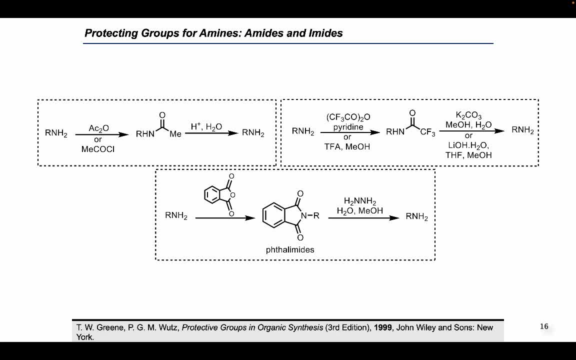 Simple amides are satisfactorily protecting microbes only if the rest of the molecule can resist the vigorous acidic or alkaline hydrolysis necessary for its removal. Otherwise, thalamides could be used for pre-protection of primary amines, as it can be cleaved by treatment with hydrazine, as in the Gabriel synthesis of amines. 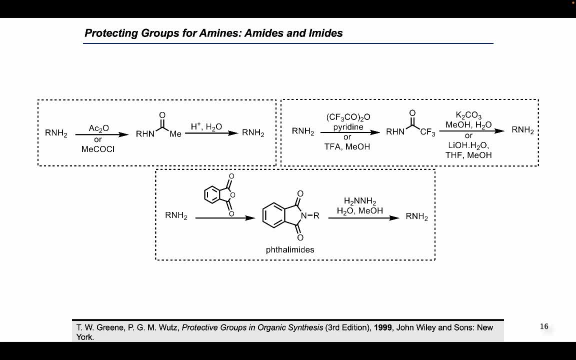 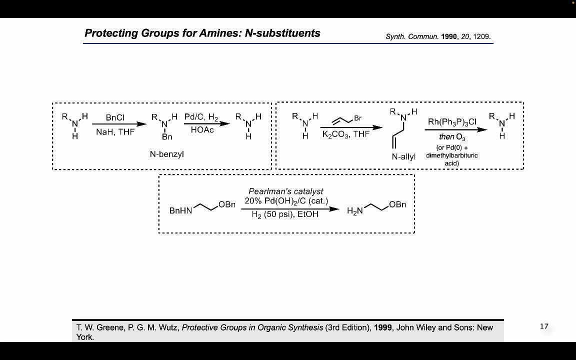 However, it does have some disadvantages. For example, it is quite sensitive to nucleophilic reagents, which, in the case of mild aqueous bases, results in ring opening. The benzyl derivative is another popular amine-protecting group, formed by the reaction of amines with benzyl chloride in presence of a base. 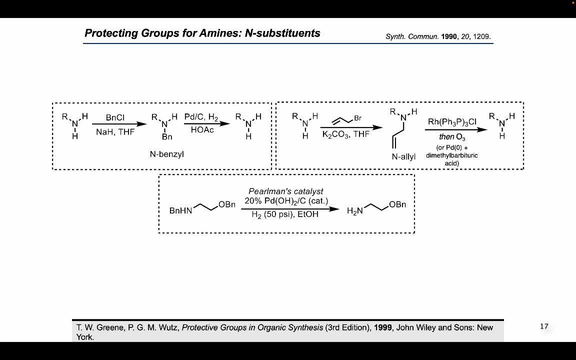 However, in some cases, dibenzylated product is obtained from the primary amines. The benzyl group is stable towards both acids and bases and can regenerate the amine by hydrogenolysis with palladium catalyst and hydrogen in presence of an acid. 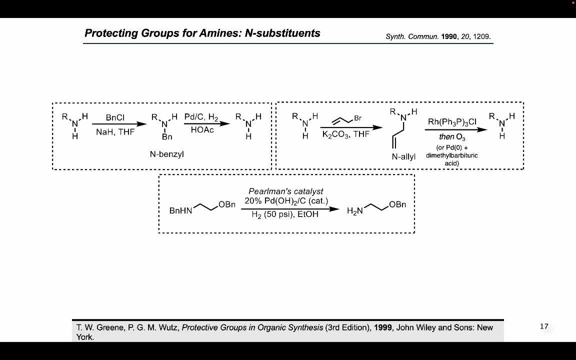 An allyl group attached directly to amine, can be removed by isomerization, and Wilkinson's catalysts have been found to be effective for the process For the selective hydrogenolysis of benzyl amines in presence of benzyl ethers, the non-pyrophoric palladium hydroxide on carbon. 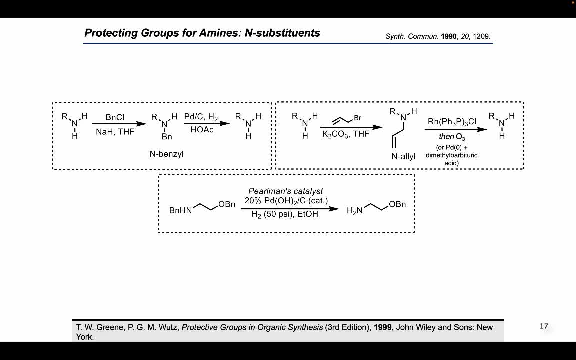 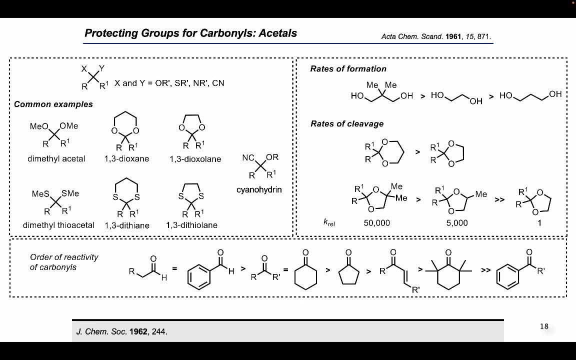 also known as the Perlman's catalyst, could be used During a synthetic sequence. a carbonyl group may have to be protected against attack by various reagents, such as strong nucleophiles, including organometallic reagents, acidic and basic conditions, or reductants and oxidants. 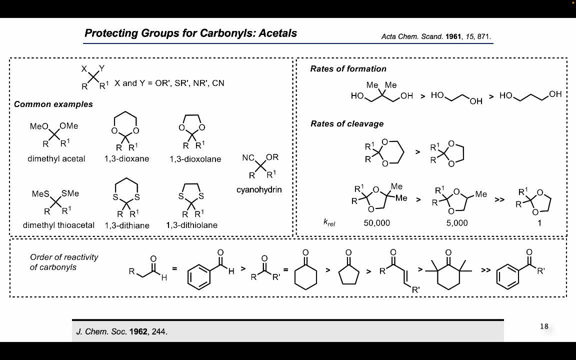 Because of the order of reactivity of a carbonyl group as shown on the present slide, it is possible to protect a reactive carbonyl group selectively in presence of a less reactive one. The most useful protective groups are the acyclic and cyclic acetone groups. 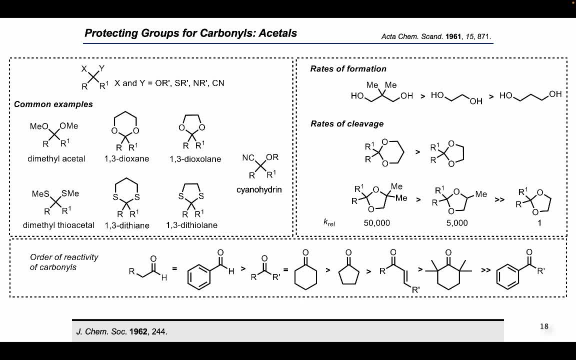 Acetyls are stable to aqueous and non-aqueous bases, to nucleophiles, including organometallic reagents, and to hydride reduction and also to most oxidants. On the other hand, a 1,3-dithiane or 1,3-dithioline, 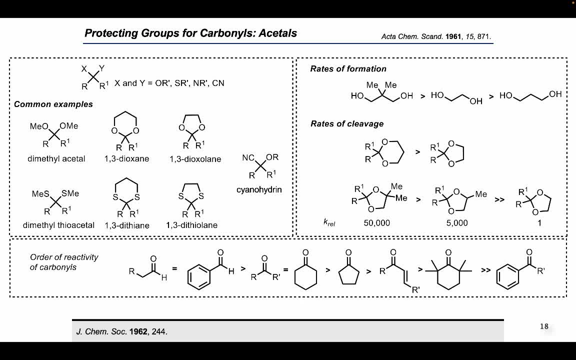 prepared to protect an aldehyde is converted to an anion when treated by a strong base such as butyllithium. On the other hand, a 1,3-dithiane or 1,3-dithioline prepared to protect an aldehyde. 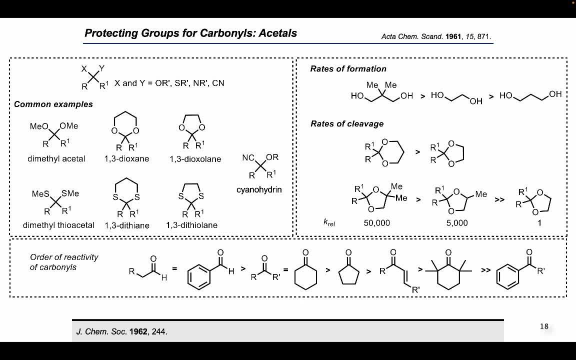 is converted to an anion when treated by a strong base such as butyllithium. Also, the sulfur analogues can be cleaved by a wide range of deductants and oxidants. The oxygen analogues, unlike the sulfur analogues. 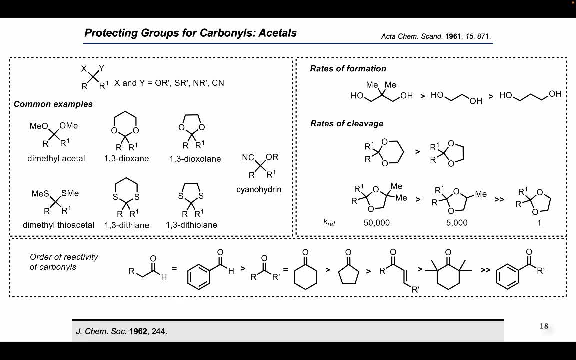 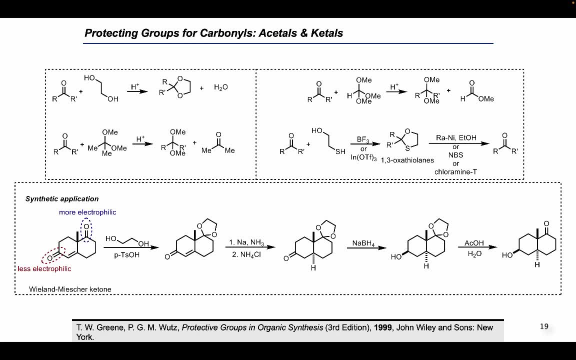 are readily cleaved by acidic hydrolysis. are readily cleaved by acidic hydrolysis. The protective group is introduced by treating the carbonyl compound in the presence of an acid with alcohol, diol, orthoester or dithiol. 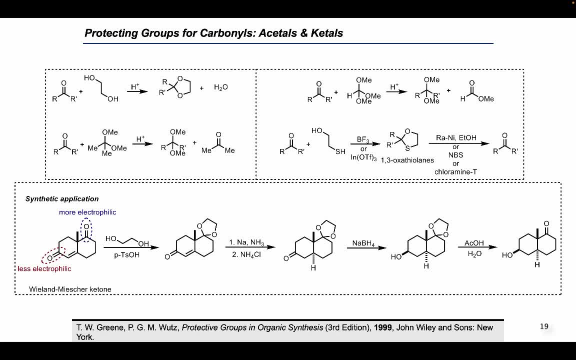 with alcohol, diol, orthoester or dithiol. Another carbonyl-protecting group is the 1,3-oxathioline derivative, which can be prepared by reaction with mercaptoethanol in presence of a lewis acid. 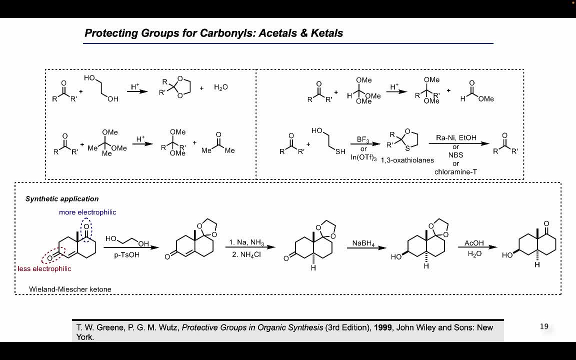 The 1,3-oxathiolines are particularly useful when non-acidic conditions are required for deprotection. The 1,3-oxathiolene group can be removed by treatment with rainy nickel in alcohol or by treating with a mild halogenating agent. 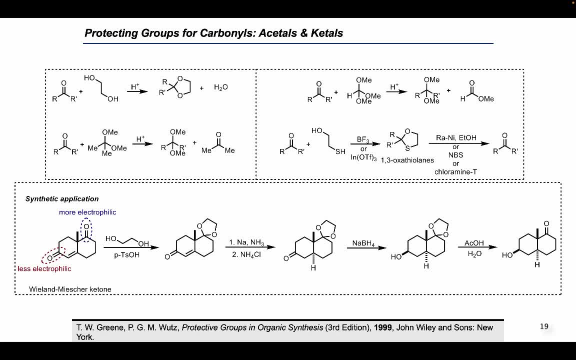 such as NBS or chloramine tea. The wieland-mischer ketone is a common intermediate in the synthesis of both natural and synthetic steroids. Because of resonance stabilization, the carbonyl of the alpha-beta unsaturated ketone is less electrophilic. 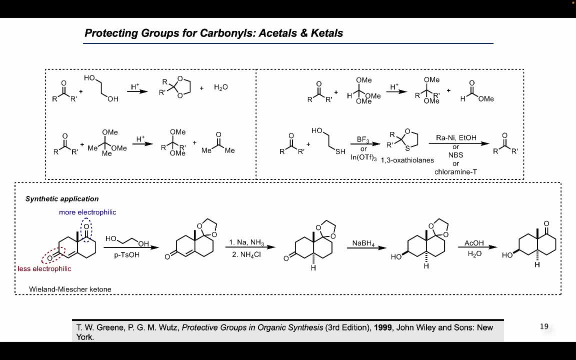 and therefore less reactive to nucleophiles compared to an isolated ketone. As a result, in order to reduce the less reactive alpha-beta unsaturated ketone, the more reactive ketone needs to be cast first. that could be done by forming a ketone by reaction. 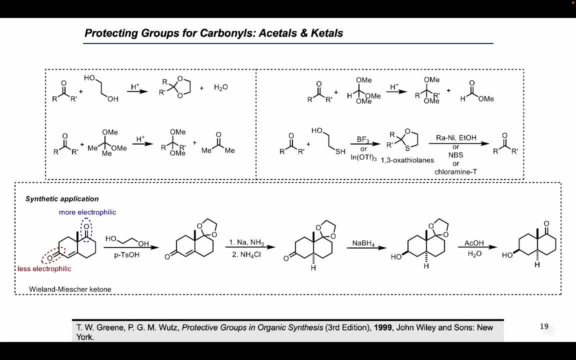 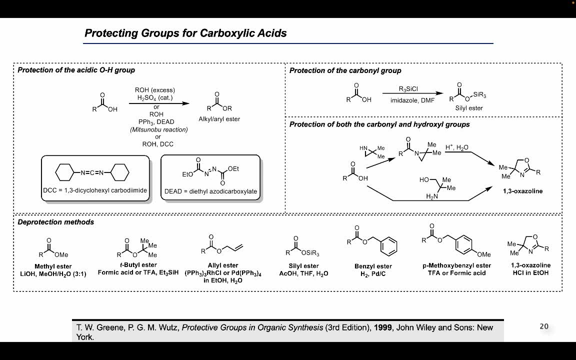 with a diol in presence of an acid. The last functional group I will talk about today is the carboxylic acids. Protecting groups for carboxylic acids are used to avoid reaction of acidic hydrogen with bases or to prevent nucleophilic. 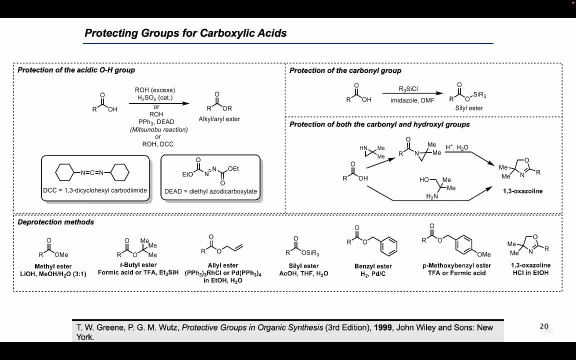 adhesion at the carbonyl group. If only the OH as opposed to the carbonyl of a carboxyl group has to be masked, it can be readily accomplished by esterification. Some of the methods for ester formation includes reaction with alcohol. 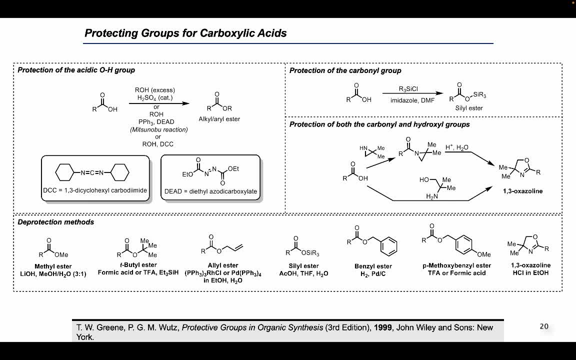 in presence of an acid or even milder condition, using DCC as the activating and dehydrating agent, or from the Mitsunobu esterification with alcohols in presence of triphenylphosphine and TED that occur under neutral conditions. 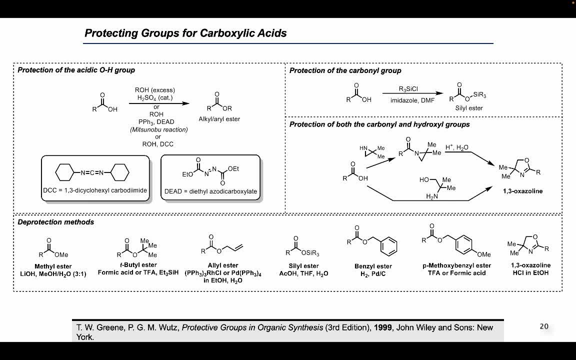 An operationally simple method for protecting the carbonyl group of COOH group against nucleophilic attack is its conversion to a silyl ester, which are cleaved by treatment with an acid. A more difficult problem of protecting both the carbonyl 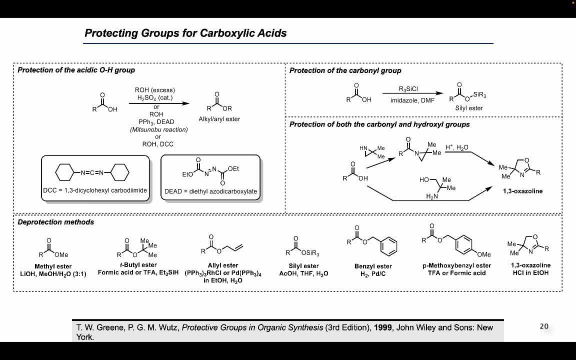 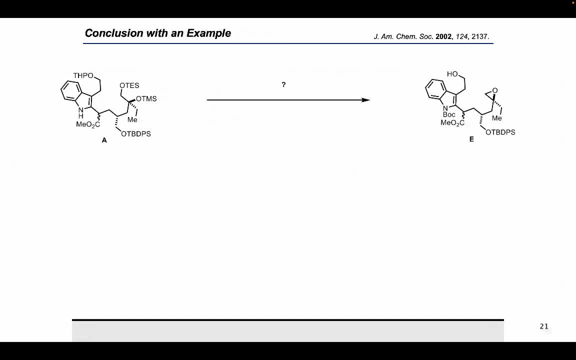 and hydroxyl group of a carboxyl group can be accomplished by conversion to an oxazoline derivative, which can be prepared from the acid by reaction with two amino to methylpropanol or with two to dimethyl aziridine. Now I would like to conclude. 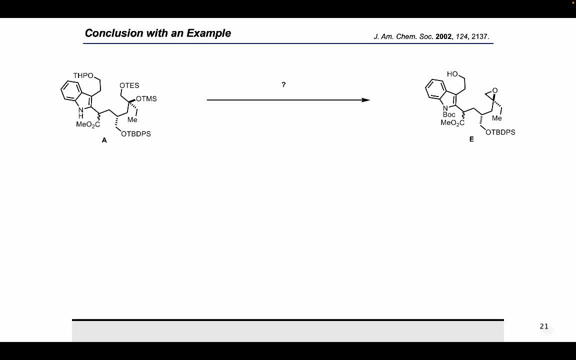 this talk with an example where we can apply the knowledge we have gained today. The question is how to convert A to E. So we start with the protection of the indole, with BOC group to get the product B. Now we have to get rid of the. 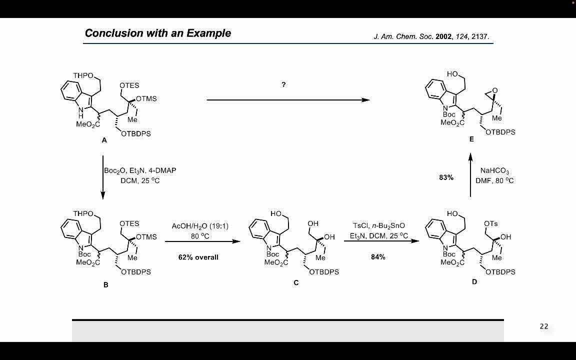 TES and TMS protecting group to form unprotected diol, which will further react to form the epoxide. Since the product E still has the TBDPS protecting group intact, we cannot use any fluoride source which is able to cleave the TBDPS group. 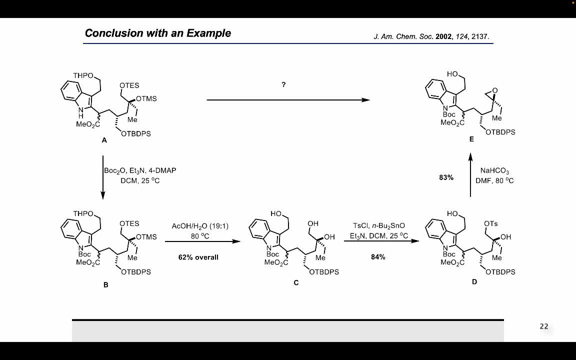 Instead, treatment with an aqueous acetic acid gives the product C in which the acid labile groups, that is, TES, TMS and THP, is cleaved, whereas the BOC group, methyl ester and bulky TBDPS protecting groups survive the condition.